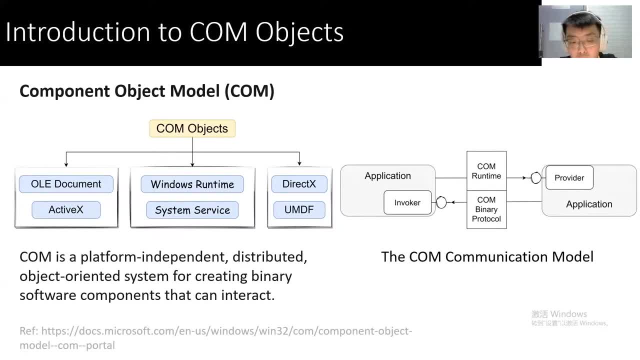 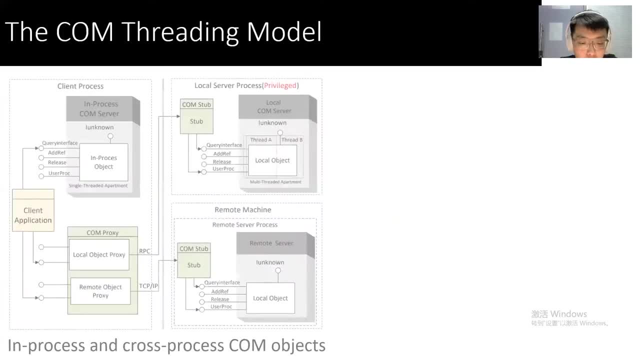 object methods via predefined interfaces through COM Runtime and Binary Protocol in which breaks the limitations and invoker and service provider need to stay in the same process. COM provides threading features, multi-threading features that course from different plans to the service object interface methods may run concurrently. COM objects use a threading. 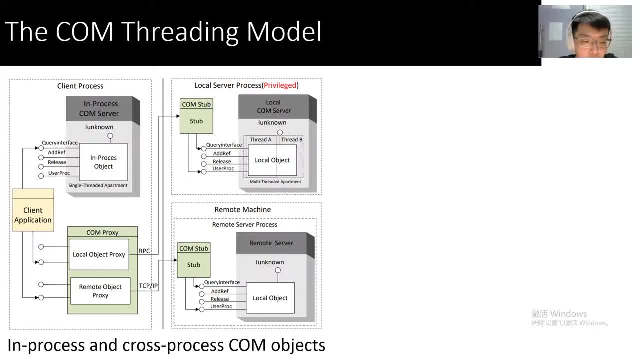 model named Apartment, which is a logical encapsulation to specify thread-sharing rules for COM objects. The left figure shows the threading model with process boundaries. There are three types of threading modes in COM. First is single-threading Apartment. A single-threading Apartment consists of: 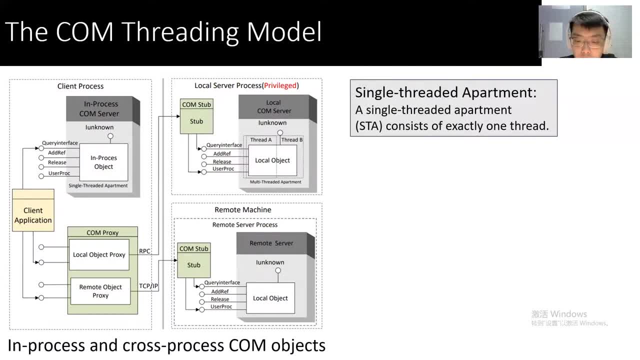 exactly one thread. A COM object in an STA can receive interface method calls from the only thread in an STA. Second is a multi-threading Apartment. A multi-threading Apartment consists of one or more threads, just as the top right corner of the picture shows. 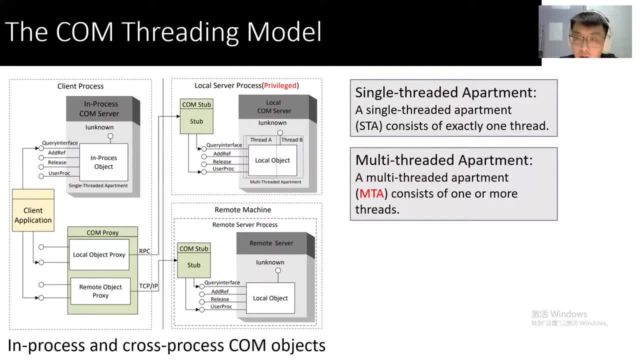 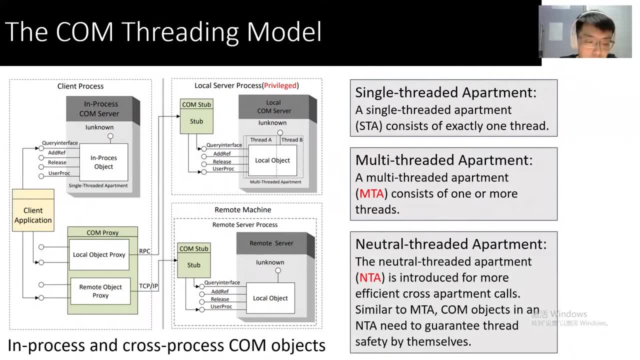 Each client request will be served with a new thread in the privileged local process. Consequently, data resets may trigger if the interface methods are not thread-safe. These data resets often lead to memory corruption bugs, such as buffer workflows and the use-after phrase. Attackers can easily exploit these bugs to gain escalated privilege or execute. 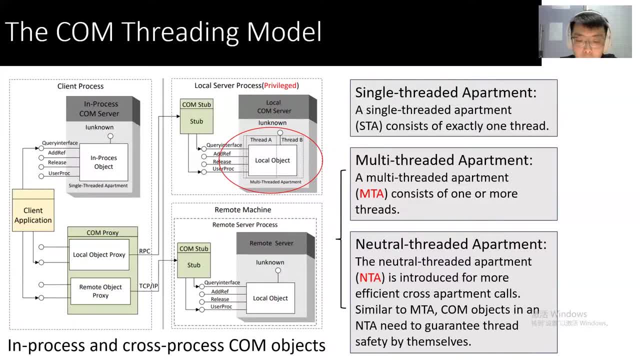 arbitrary code. Third is a neutral threading department. The neutral threading department is introduced for a more efficient host-apartment course, Similar to MTA. COM objects in an MTA need to guarantee thread-safe by themselves. Our research found out that MTA and 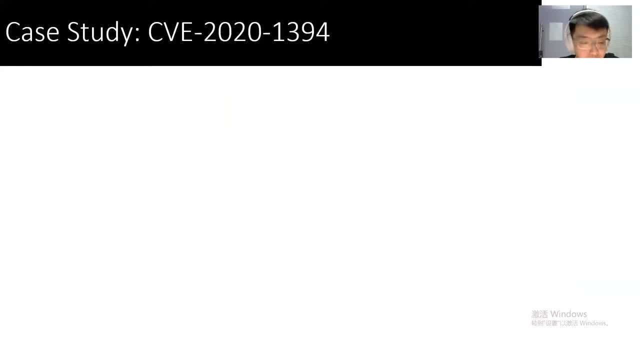 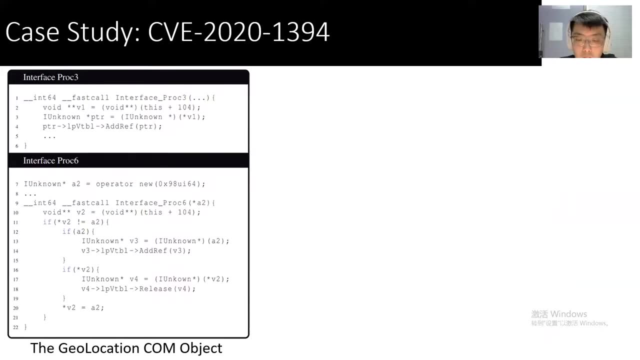 COM objects are prone to data reset attacks if thread safety is not guaranteed. We demonstrate the real-world data resets in a geolocation COM object which is acting as a system service object running inside the service host process. The left picture shows the decompilation code of two interface methods of the object: The interface method proc3 and proc6. 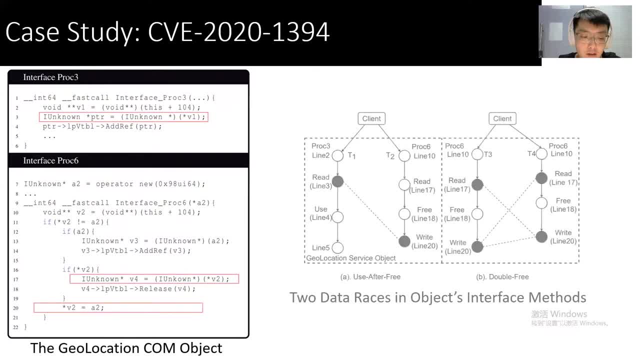 introduce two high-impact model bases of the object. As the red figure shows, if the client invokes methods 3 and 6 concurrently, since proc3 and proc6 are methods of the same object, the object's geolocation is the same as the object's geolocation, The land. 3 of proc3 and. 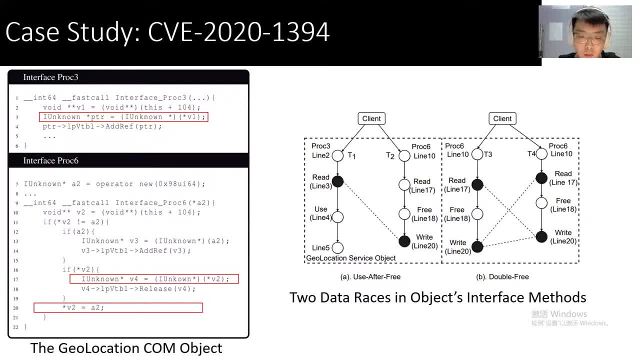 land 20 of proc6 operates similarly. The former is readout and the latter is read-to. In the meantime, proc6 freezes plus 104 at land 18, which results in a possible use-after free vulnerability while invoking proc3 and proc6 concurrently. Similar things happen when clients invoke proc6 alone. 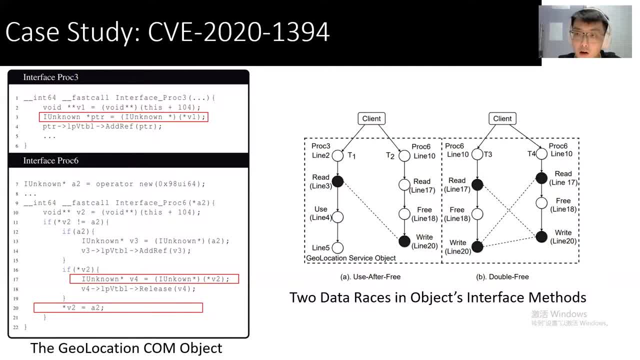 If one free operation at land 18 happens before another free operation in another service thread, proc6, free will happen. The two subsets tend mostly to privilege hesitation. in this scenario, In order to effectively detect data risk problems in the large size of COM boundaries in the 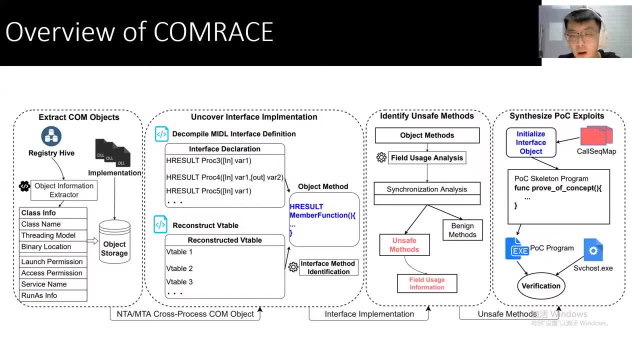 underlying system. we propose a static solution named comrace. comrace solves the problem in four steps: Extract COM objects, uncover interface information, identify unsafe methods and synthesize PoC exploits. Firstly, we extract COM object information and solve them locally. 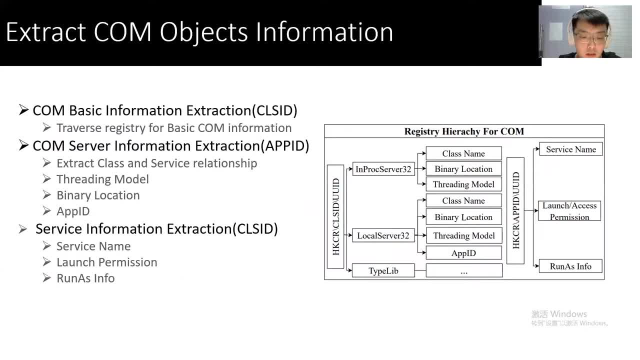 which is the basic step of the solution. COM object thread restarts themselves under the Windows registry path hk-classes-root-class-id, with a unique CRS ID so we can extract information needed from the registry. comrace extracts COM class information, including basic information, then it extracts service information and service information. 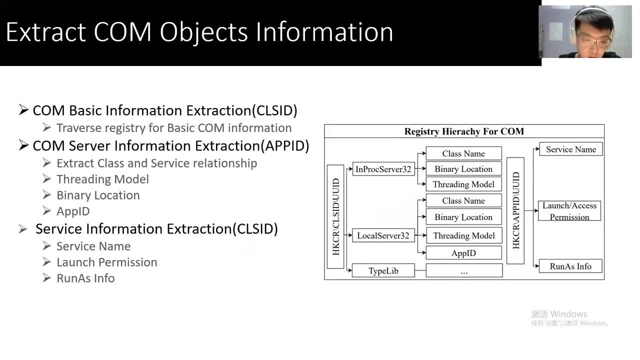 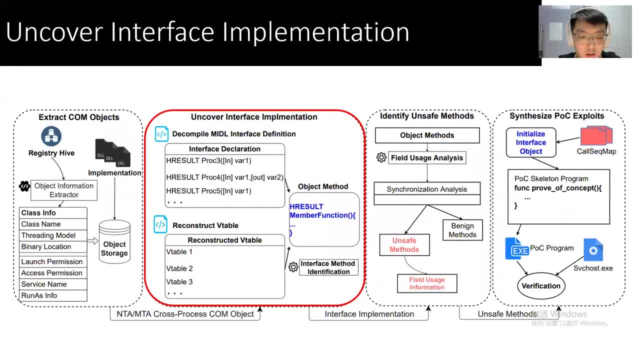 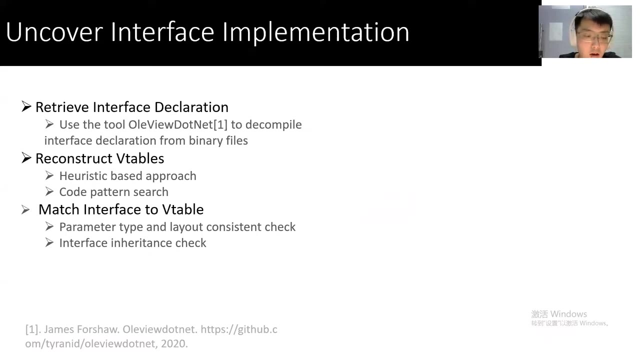 After this step, comrace gets registered COM's: class name, thread model, binary, location, service permissions and so on. After extracting the information of COM objects, we dig into the COM object implementation binary to uncover interface implementation. COM exposes interface implemented in its corresponding binary file: The implementation of an interface method. 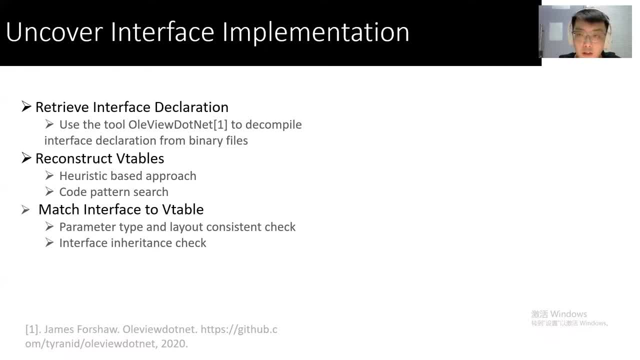 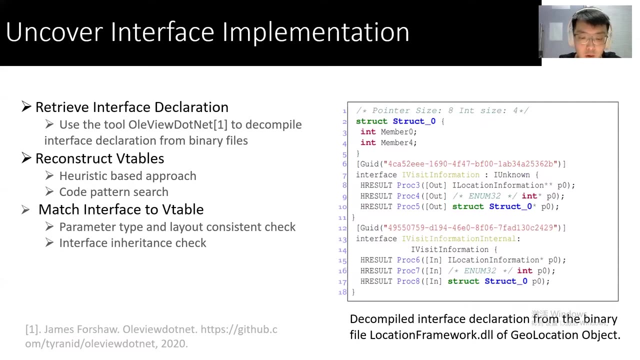 has exactly the same type signature as the interface declaration. Firstly, comrace needs to retrieve the interface declaration from binary files. This process is completed with the help of oreviewnet. The decompiled geolocation interface is shown on the right. Secondly, in order to locate the right implementation of the COM object. 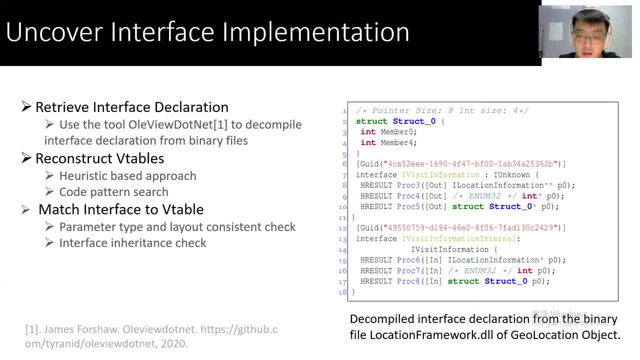 we need to reconstruct vtable information from the binary. The vtable reconstruct procedure relies on three key observations of the Windows binaries. We use observations and heuristic rules for guiding vtable reconstruction procedure. After uncovering the vtables and interface declarations, we try to find the vtables and implement all declared interface methods. This can be. 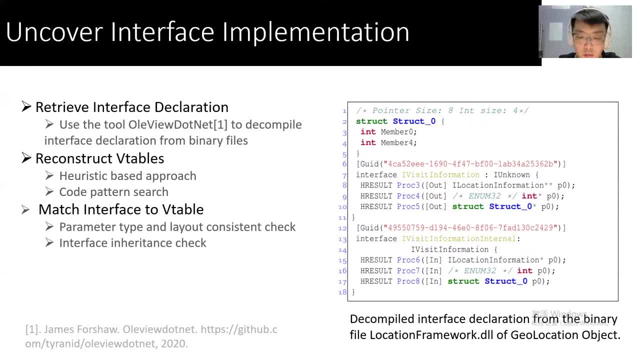 challenging, since we lost method names and user-defined structure information. For every vtable candidate, we firstly examine the parameter type and the interface layout consistently, After which candidate lists shrink to those interfaces as inheritance relationships. We design an interface inheritance check to select the corresponding vtable which indicates: 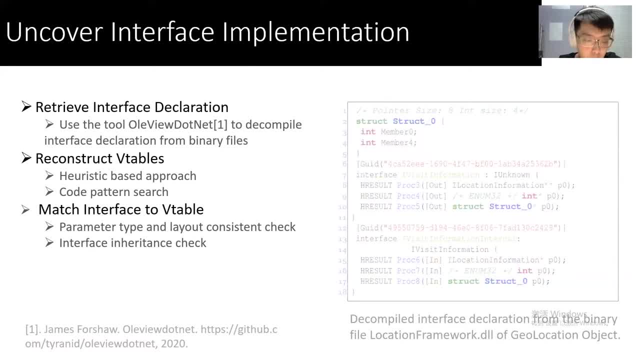 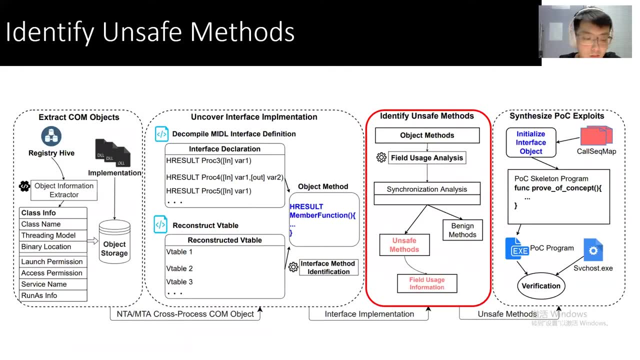 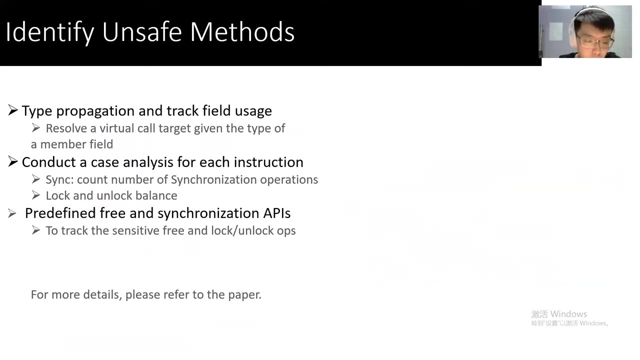 the corresponding interface implementation. Now we have the corresponding implementation of each interface method. We can identify unsafe methods. An interface method is regarded as unsafe if it can access member fields without its synchronization. Hence we examine every instruction interface method, as well as its calling methods, to check. 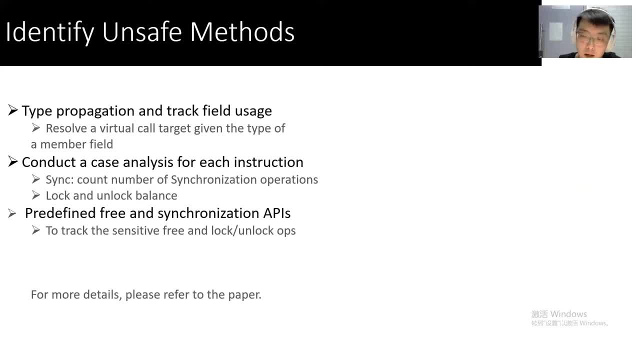 whether there exists an unguarded field access or not. This is realized by shrunking the usage of this pointer, since all member fields are accessed via this pointer with constant offsets. This module reports all unsafe methods and unguarded field offsets with six types. 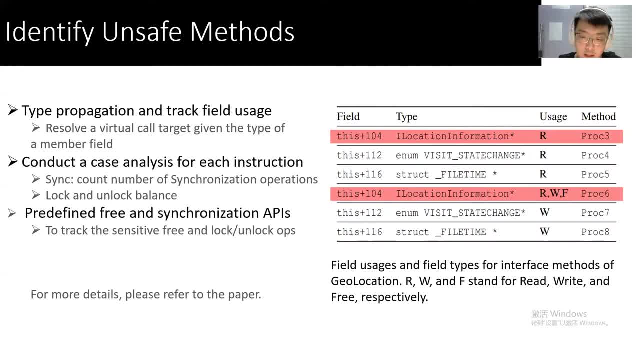 read-read, read-write, read-free, write-write, write-free and free-free resets. An example of the analyzed field usage and field types for interface methods of geo locations shown at the right picture. The most important part of our algorithm is processing virtual method invocations. 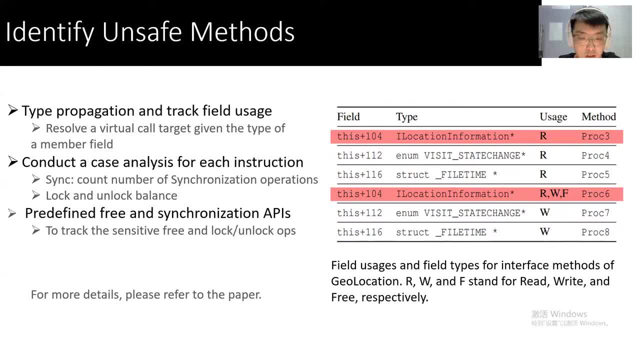 We apply the type propagation method and the track field usage to resolve a virtual call target given the type of the member field. And then we conduct case analysis for each instruction. We define a sync variable to count the number of synchronization operations, to check if lock and un-lock. 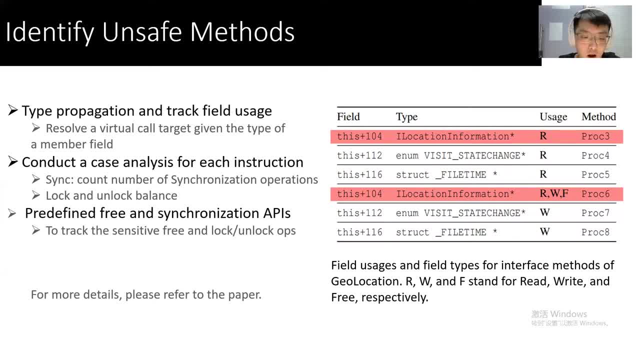 operations are balanced. we also applied a list of predefined free and synchronization APIs to train the sensitive free and lock-on-lock operations. For more details, please refer to our paper. In order to verify the output of identified unsafe methods, Comrace appends a module to 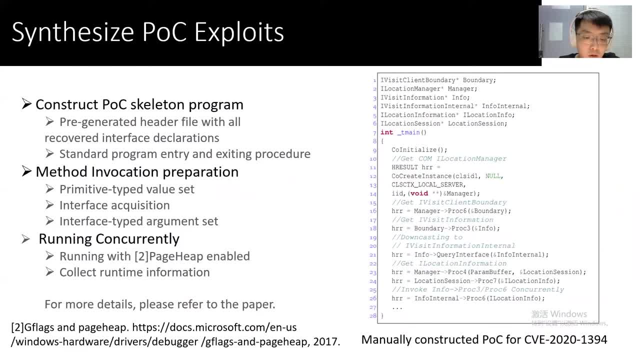 try to synthesize POC exploits automatically. The POC synthesizers are built on a predefined POC skeleton program. This is because the POC programs share a similarity to a certain extent. A manual program for the example, CVE, is shown at the right picture. 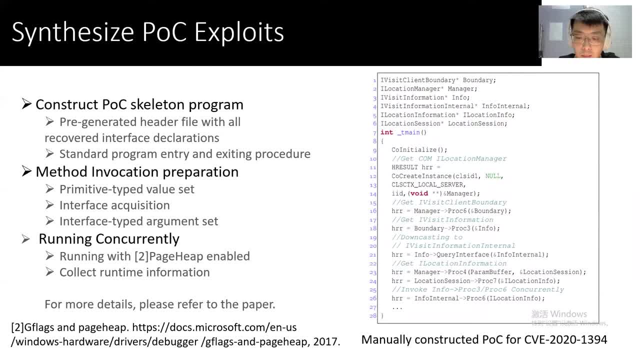 The POC skeleton program uses a pre-generated header file to complete the variable definition part as the first red cube. Now the key problem is now how to prepare parameter values for the interface method. For primitive values, we set random chosen initial value. For interface-type values, we traverse interface dependency graphs to generate a sequence of 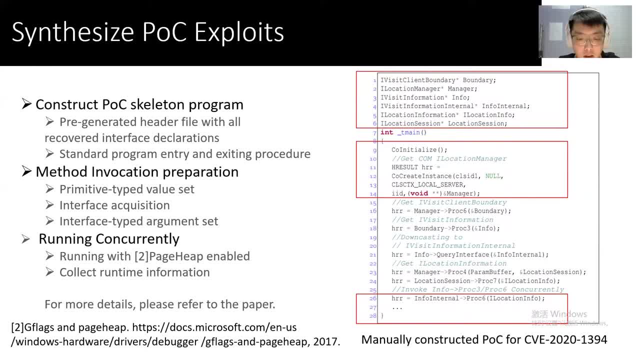 method ports to get the interface-type arguments in place. Then, after the POC program compiled, we run the POC program concurrently with PHP enabled and collect runtime information. Evaluation: We evaluated the effectiveness of Comrace on Windows operating systems and the ReactOS. 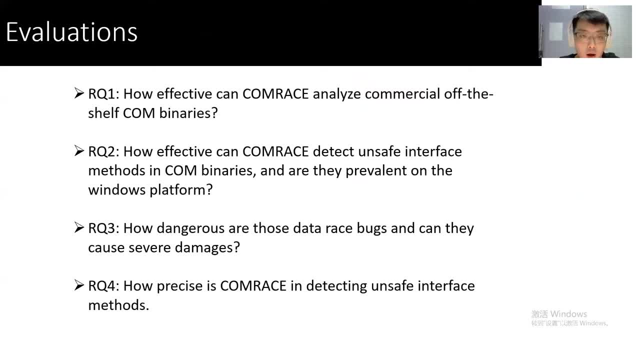 system. We designed several experiments to answer the following questions. Question 1. How effectively can Comrace analyze commercial office shell combineries? Question 2. How effectively can Comrace detect unsafe interface methods in combineries? Question 3. How effectively can Comrace detect unsafe interface methods in combineries? 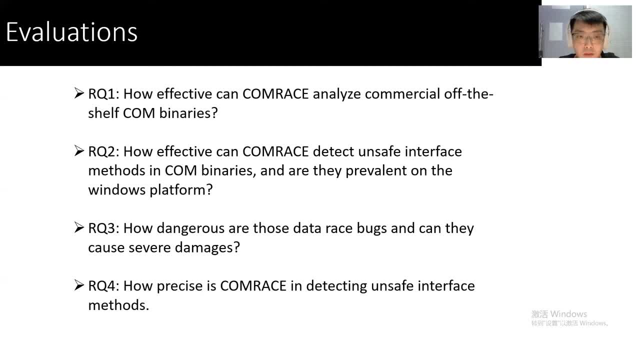 Question 4.. How effectively can Comrace analyze commercial office shell combineries? Question 5.. Are they prevalent on the Windows platform? Question 6.. How dangerous are those data risks bugs and can they cause severe damages? Question 7.. 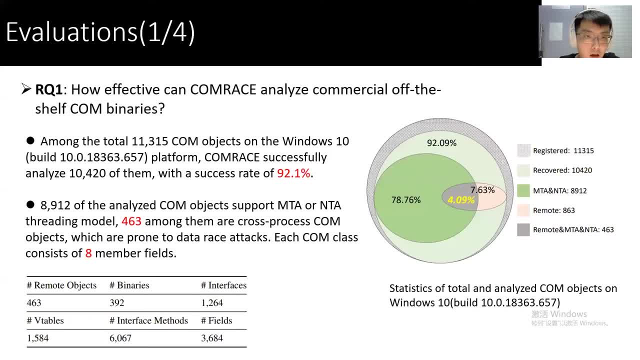 How precise is Comrace in detecting unsafe interface methods? Question 8.. For the first question, how effectively can Comrace analyze commercial office shell combineries? Among the total combo objects on the Windows 10 platform, Comrace successfully analyzed 10420 of them, with a success rate of 92.1%. 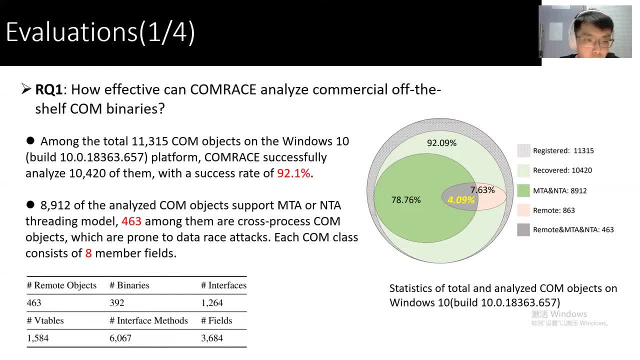 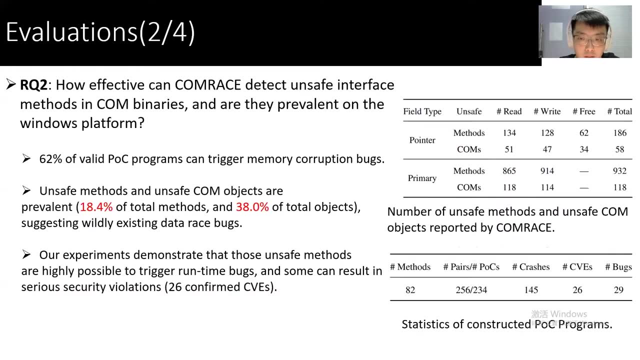 Question 9.. Are there more than 80,000 of the analyzed combiners that support MTA or MTA threading model? 463 among them are post-processed com objects which are prone to data-risk attacks. Each com class consists of eight member fields on average. 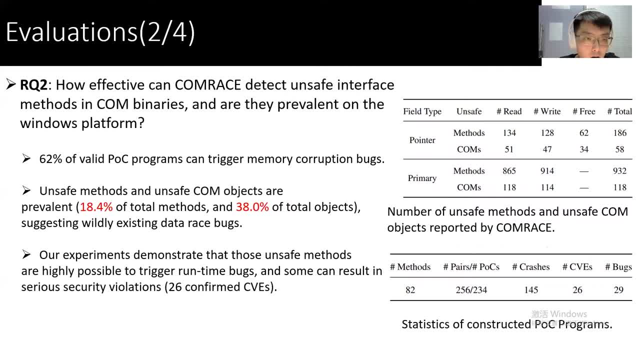 Question 10.. For the second question: how effective can Comrace detect unsafe interface methods in combineries? Are they prevalent on the Windows горbe platform? Question 11, how are these Negro drone tests safe? How effective can Comrace detect unsafe interface methods in combineries and are they prevalent? 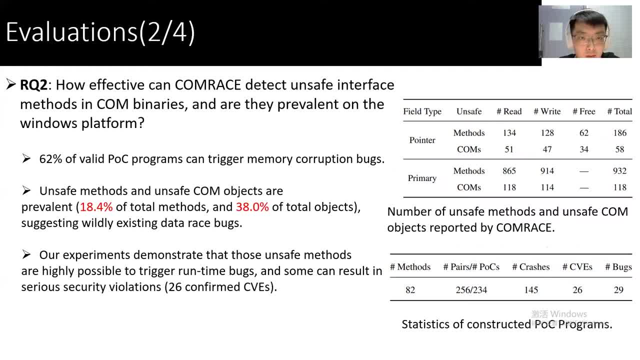 on the Windows platform, 62% of the valid QC programs can trigger memory question bugs. Unsafe methods and unsafe combat objects are prevalent: 18.4% of total methods and 38% of total objects, suggesting widely existing data risk bugs. Our experiment demonstrates that those unsafe methods are highly possible to trigger runtime bugs. 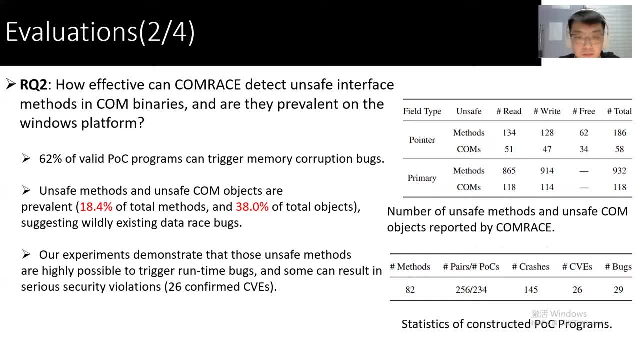 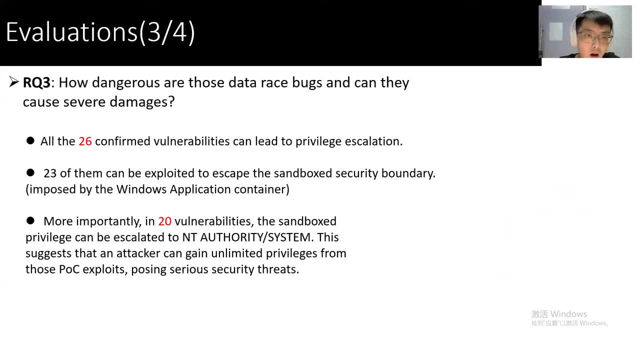 and some can result in serious security violations. Question 3. How dangerous are those data risk bugs and can they cause severe damages? All the 26 confirmed vulnerabilities can lead to privilege escalation. 23 of them can be exploited to escape the sandbox security boundary imposed by the Windows application container. 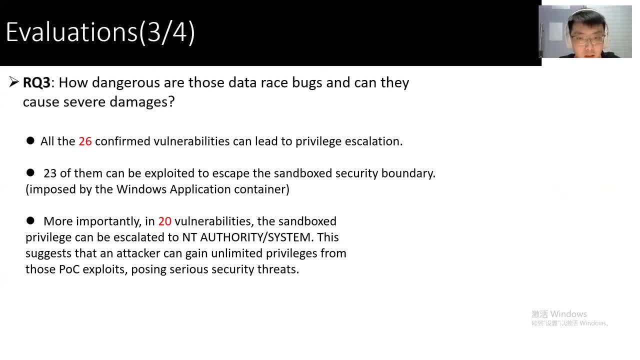 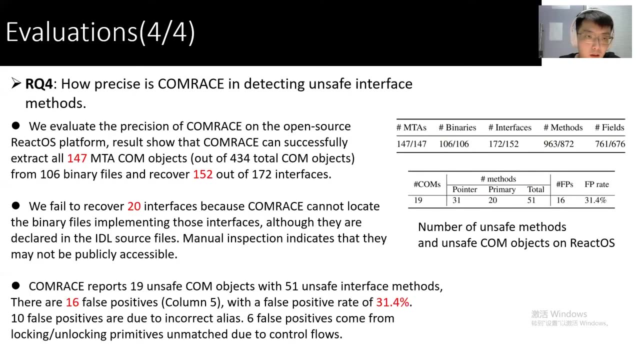 More importantly, in 20 vulnerabilities the sandboxed privilege can be explained to an anti-authority system. This suggests that an attacker can gain unlimited privileges from those QC exploits posing serious security threats. Question 4. How precise is Comrace in detecting unsafe interface methods? 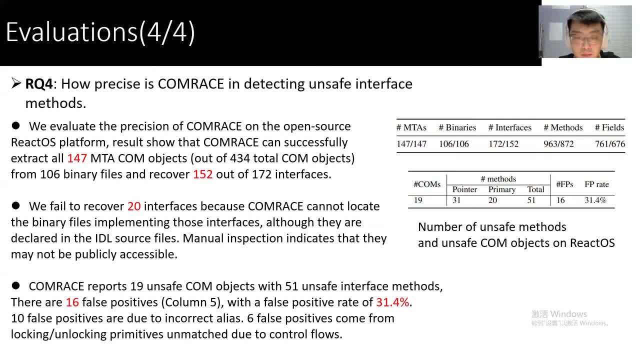 We evaluated the precision of Comrace on the open-source ReactOS platform. Results show that Comrace can successfully extract all 147 MTA COM objects, auto 434 total COM objects from 100 binary fields and recover 152 auto COM objects. 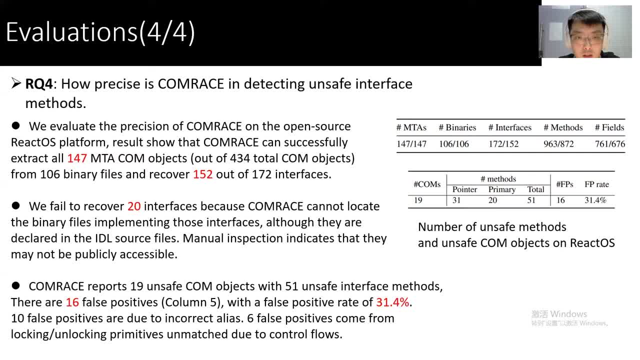 The field tool recovered 20 interfaces. because Comrace cannot locate the binary field implementing those interfaces. although they are declared in the ideal source files, Manual inspection indicates that they may not be publicly accessible. Comrace reports 19 unsafe COM objects with 51 unsafe interface methods. 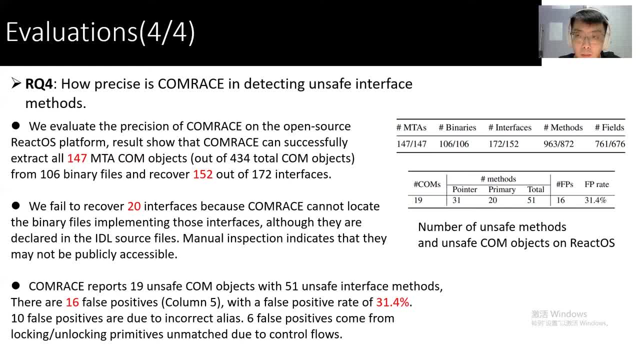 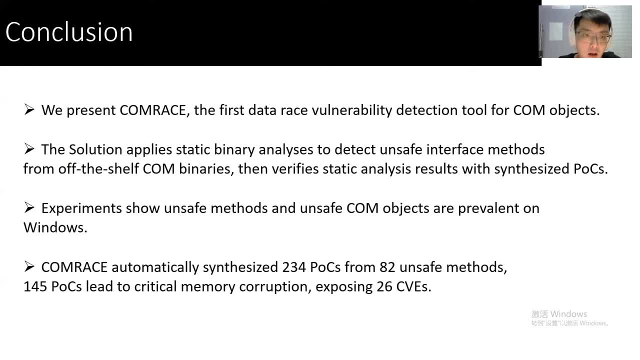 These are 16 false positives with a false hit rate of 31.4%. Conclusion: With present Comrace, the first data risk vulnerability detection method is the detection tool for COM objects. The solution applies static binary access to detect unsafe methods from the off-the-shelf binaries. 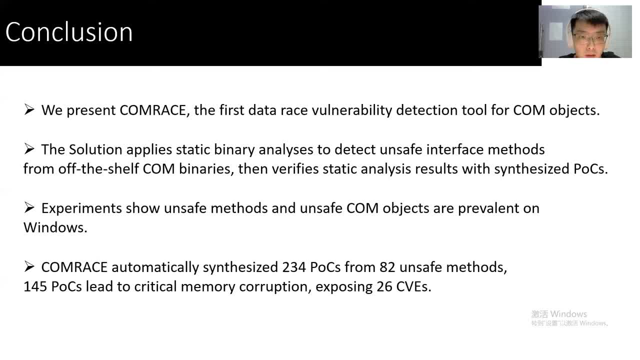 then verifies static analysis results with synthesized POCs. Experiments show that unsafe methods and unsafe COM objects are prevalent on Windows. Comrace automatically synthesized 234 POCs from 82 unsafe methods. 145 POCs lead to critical memory co-options. 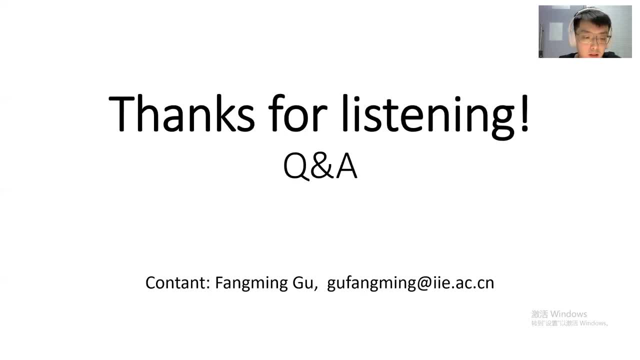 exposing 26 CVEs. This is it for my talk. Thanks for listening. Questions are welcome.